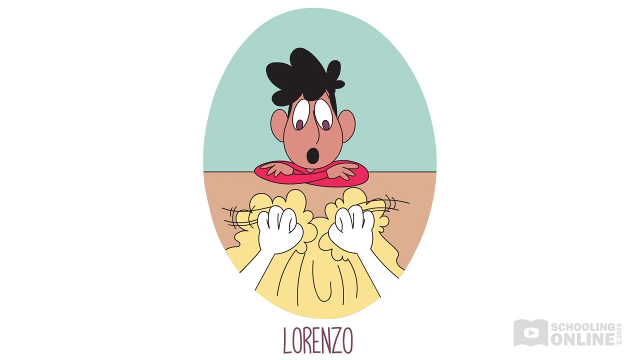 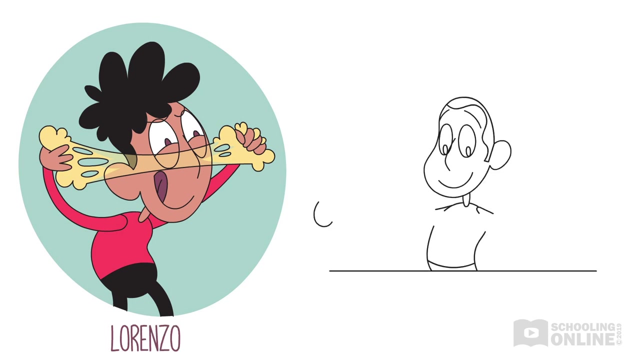 Lorenzo watches his dad with great interest. He's making pasta dough, pushing and pulling it, rolling it and pounding it with his fists. That's one long gooey mess. Dad laughs, Lorenzo, Lorenzo's dad chuckles. You know, son, when I push or pull the dough, I'm using force to change the shape of what I'm holding. 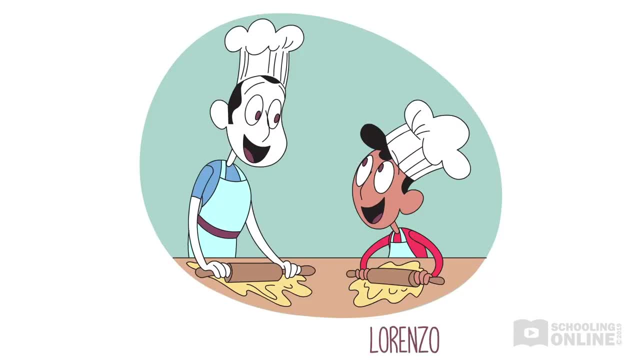 Now pay attention while I show you how to do different, even special, things with my dough. Grab your kitchen stool, son. We're going to make linguine, says his dad. Lorenzo grabs his stool and pushes it up to the kitchen bench. 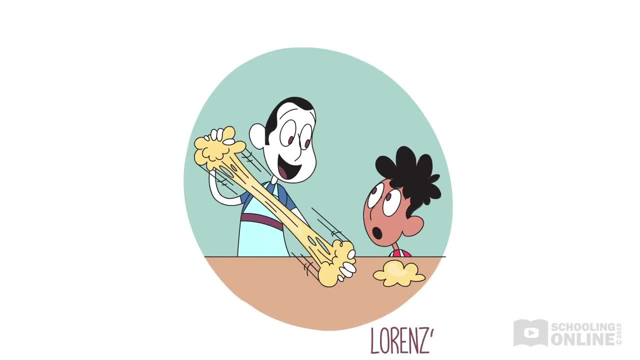 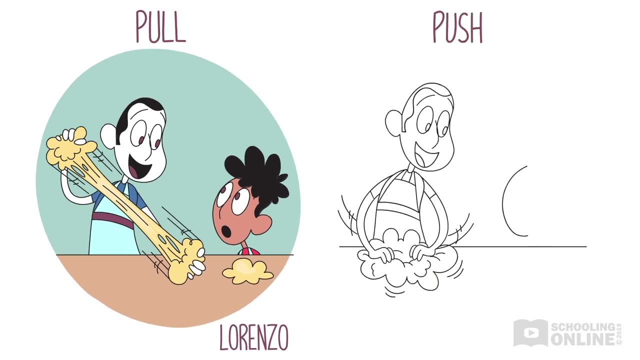 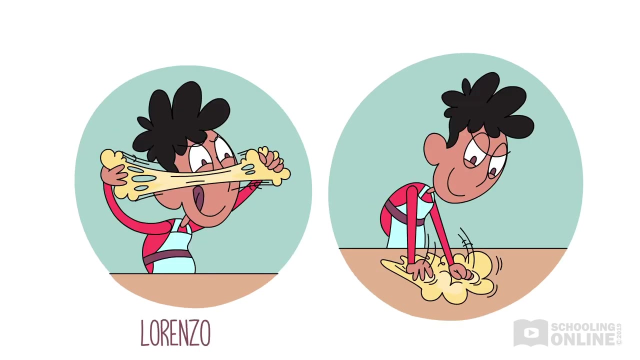 What's first, Dad? First we pull and stretch the dough, Then we push and squish the dough, explains Lorenzo's dad. Lorenzo copies his dad pulling and pushing a piece of dough in his hands, watching it change from a round blob shape to a long, thin shape. 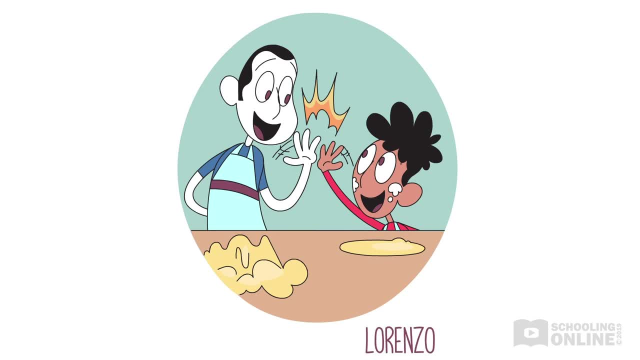 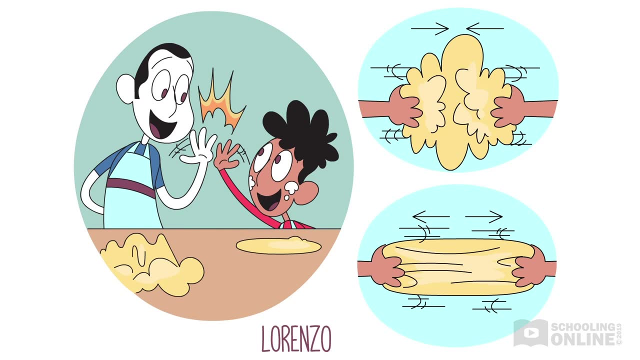 Good boy, Lorenzo. You're putting force on the pasta dough by pushing and pulling it with your hands. The force is changing its shape. Have you noticed, Lorenzo, that the harder you pull the dough, the more it changes shape? Lorenzo nods. 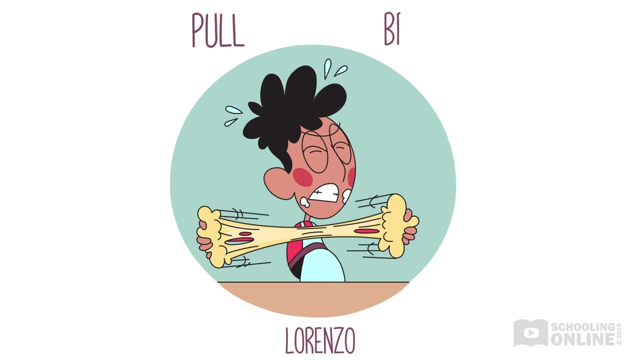 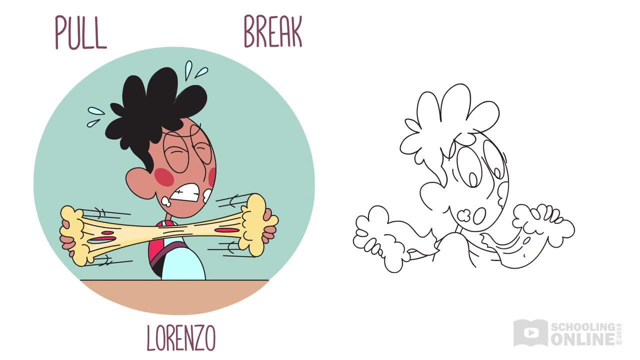 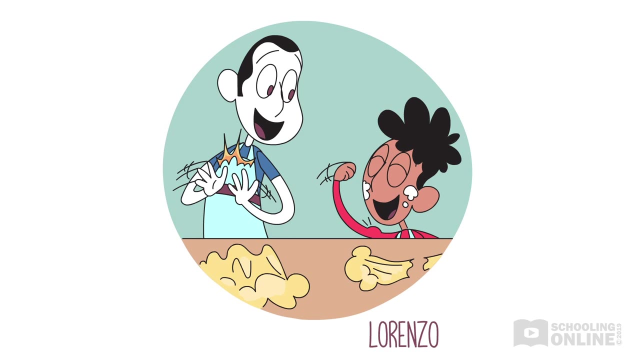 Do you think you can pull it hard enough to make it break? Lorenzo pulls and pulls his dough. It stretches and stretches until suddenly it breaks. What a strong lad you are. commences, dad. Now comes the fun part: making the pasta. 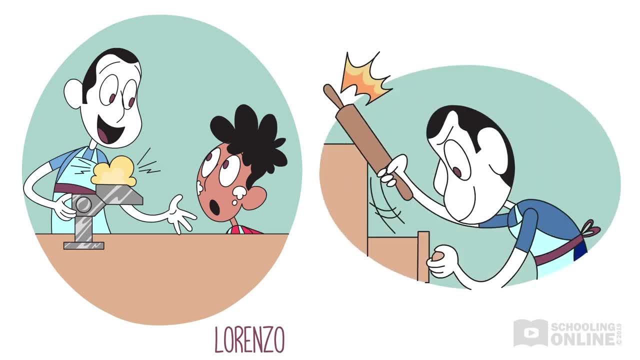 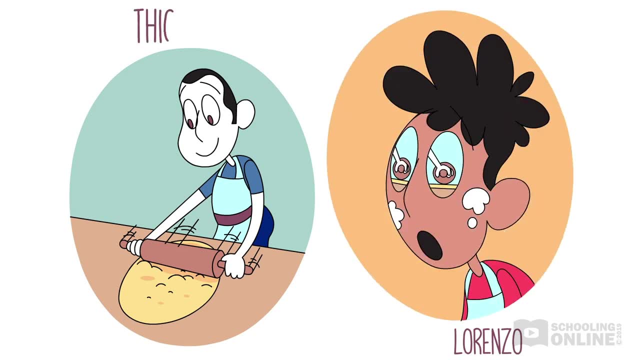 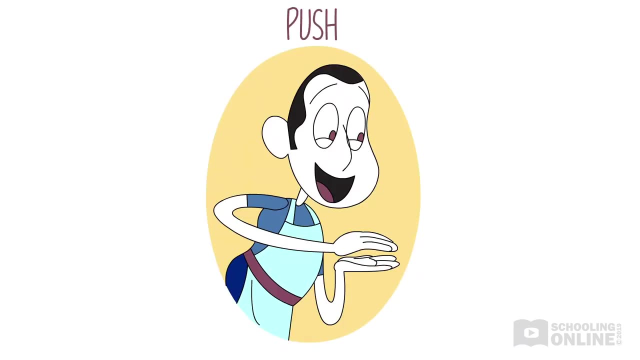 First we'll need to roll the dough out a bit with a rolling pin. Back and forth, he rolls it, spreading the dough out into a thick oval shape. I can't push as hard on this dough as the pasta machine can, even though I am. 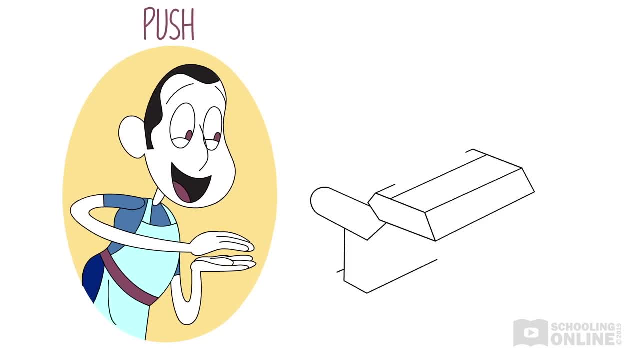 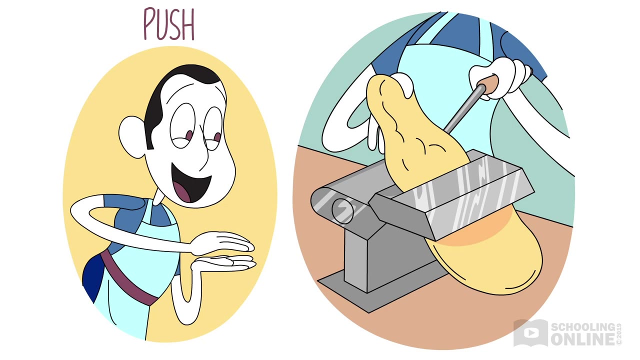 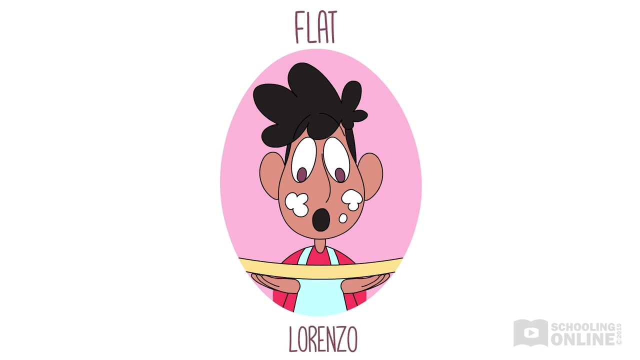 a very strong man. Lorenzo's dad slowly feeds the thick, oval-shaped dough into the pasta machine's rollers and starts turning the handle. It comes out long, wide and flat. The machine has stretched out the dough. Wow, gasps, Lorenzo, It's completely flat. It is very flat, but it's not quite thin.